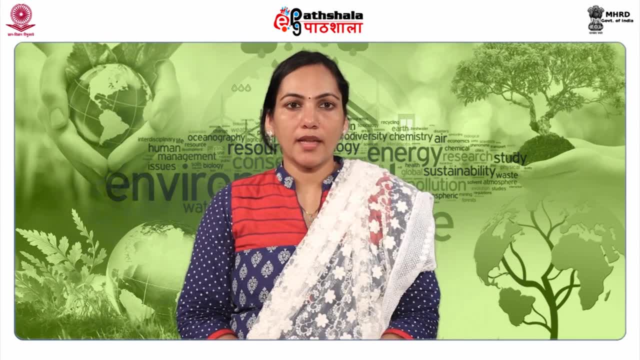 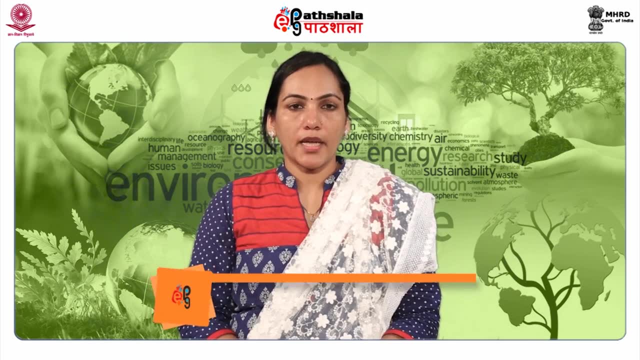 circulation and distribution, their physical and chemical properties and their reaction with the environment, including their relationship with the environment. their physical and chemical properties and their reaction with the environment, including their reaction with the environment, including their relation to living things, The entire living world of our planet, that is, the plants. 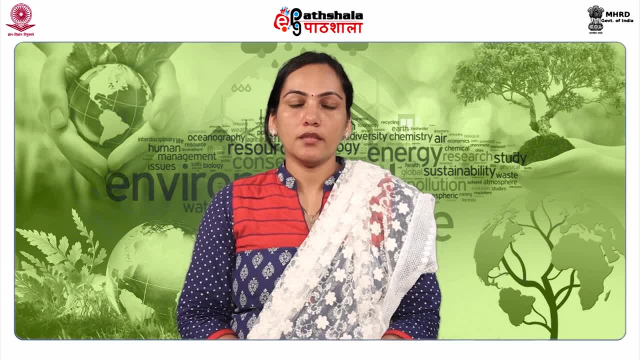 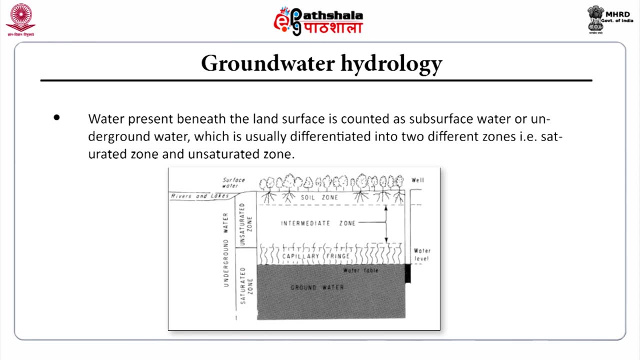 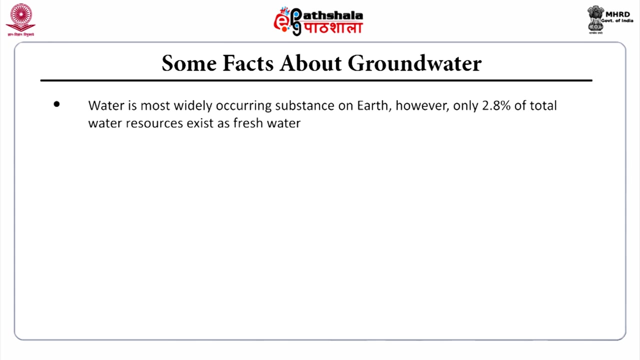 animals and human beings depend upon water for their survival. Water present beneath the land surface is counted as surface water or underground water, which is usually differentiated into two different zones: saturated zone and unsaturated zone, as shown in this figure. Some facts about groundwater. Water is most widely occurring substance on earth, However, only 2.8 percent. 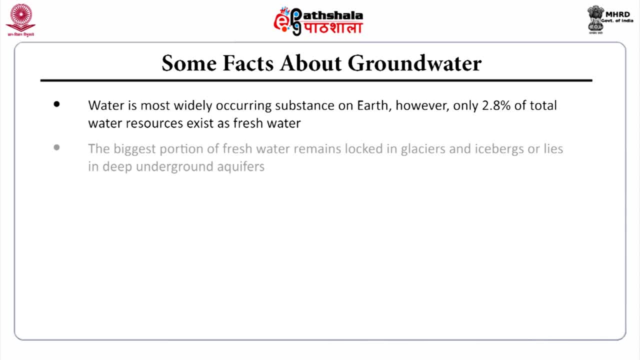 of total water resources exist as fresh water. The biggest portion of fresh water remains locked in glaciers and icebergs or lies in deep underground aquifers. Out of this 2.8 percent, about 0.6 percent is available as groundwater and only 0.3 percent can be extracted. 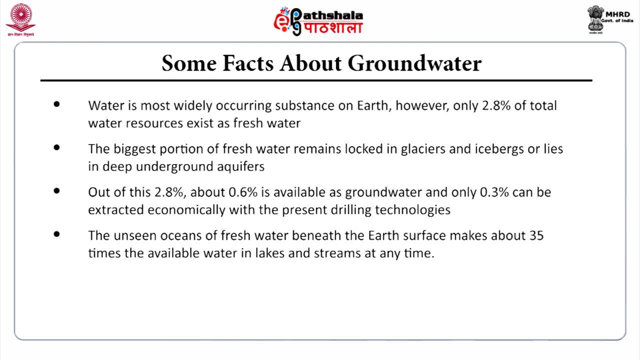 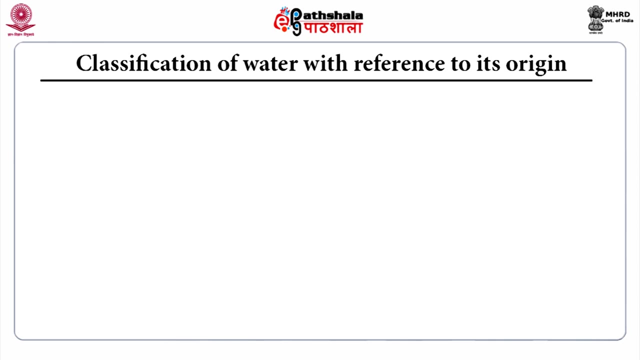 economically with the present drilling technologies. The unseen oceans of fresh water beneath the earth's surface makes about 35 times the available water in lakes and streams at any time. The available groundwater for human consumption generally occurs within 800 meters from the earth's surface. Now the classification of water with reference to its origin. Most of 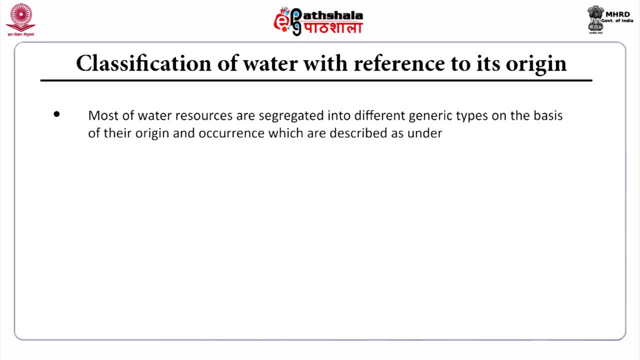 the water resources are segregated from the earth's surface. The classification of water with reference to its origin is classified into different generic types on the basis of their origin and occurrence, which are described as: under Magnetic water, The occurrence of water within and in equilibrium with a magma, or water rich volatile fluids derived from a magma. 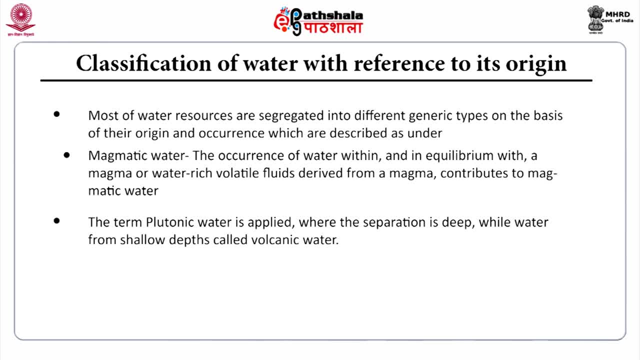 contributes to magmatic water. The term plutonic water is applied where the separation is deep, called volcanic water, juvenile water- This form of water is also known as new water, which has not been introduced to hydrosphere previously, Meteoric water. most of the 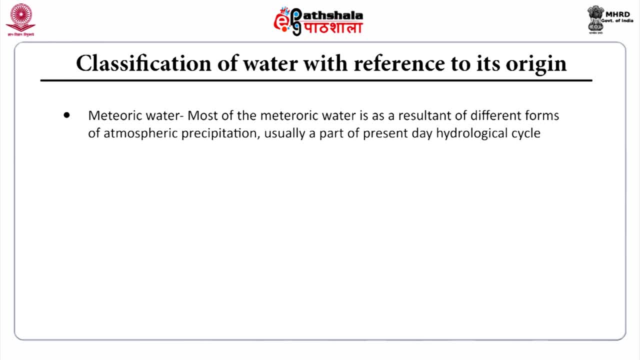 meteoric water is, as a resultant of different forms of atmospheric precipitation, usually a part of present day hydrological cycle. This resource facilitates the water available in lakes, rivers, streams, wells and ice melts, which originates directly or indirectly from the precipitation. Conate water, the water retained in ancient aquifers encountered. 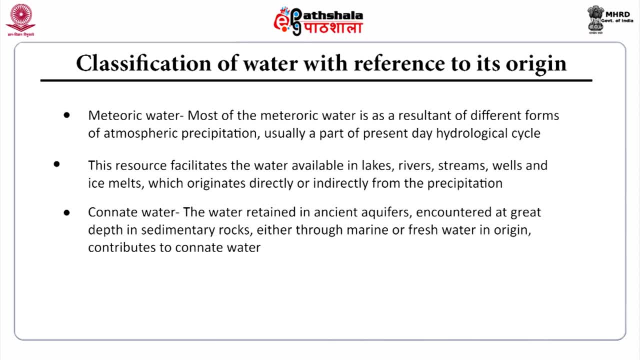 as great depth in sedimentary rocks, either through marine or fresh water in origin, contributes to conate water, Then metamorphic water. this term is used for water associated with the water in the water. This term is used for water associated with the water in the water. water in the water. This term is used for water associated with the water in the water. This term is used for water associated with the water in the water. water in the water. This term is used for water associated with the water in the water. water in the water. This term is used for water associated. 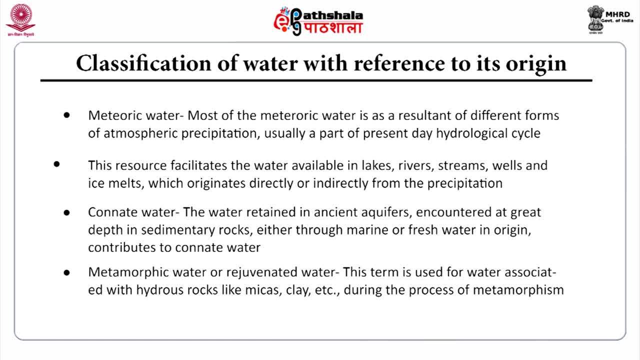 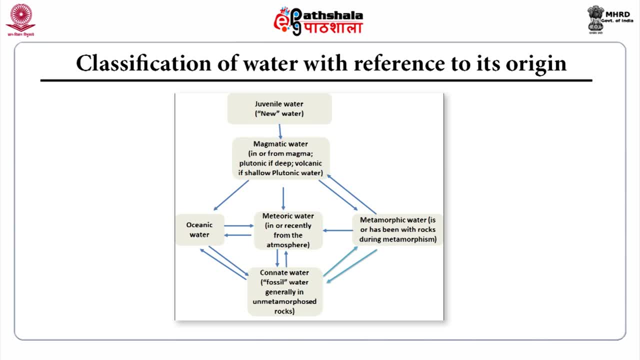 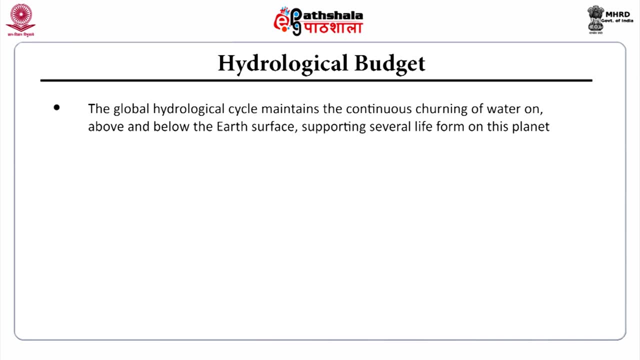 with hydrous rocks like micas, clay, etc. during the process of metamorphism. This figure shows how these different kinds of waters are interrelated to each other. Hydrological budget- the global hydrological cycle maintains the continuous churning of water on above and below. 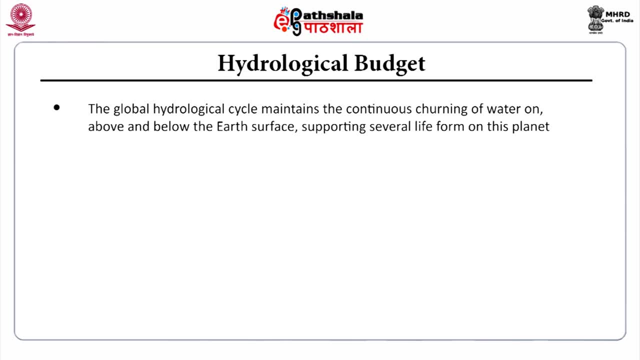 the Earth's surface, supporting several life forms on this planet. The system can be subdivided using usually into three different subsystems: atmospheric water system, surface water system and subsurface water system. The atmospheric system includes precipitation, evaporation, interception and transpiration. 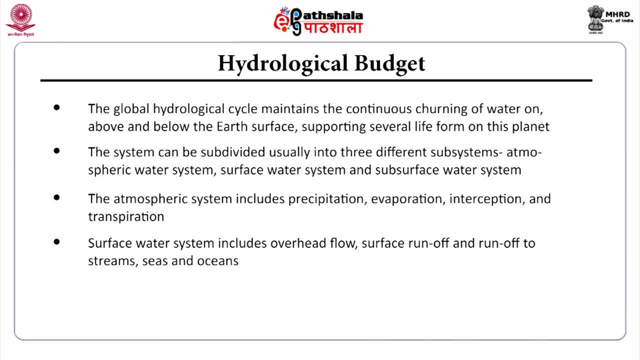 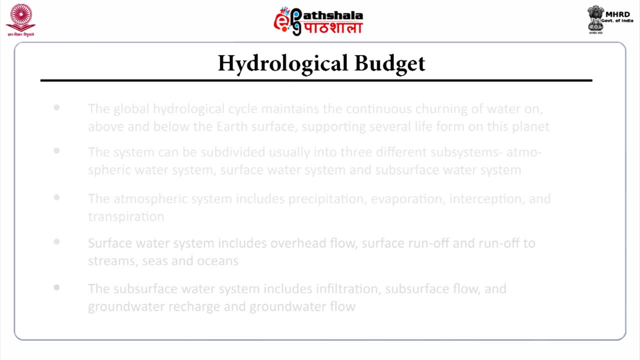 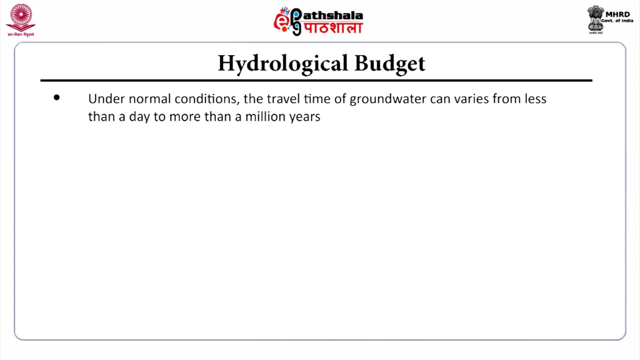 Surface water system includes overhead flow, surface runoff and runoff to streams, seas and oceans. The subsurface water system includes infiltration, subsurface flow and groundwater recharge and groundwater flow. Under normal conditions, the travel time of groundwater can varies from less than a day. 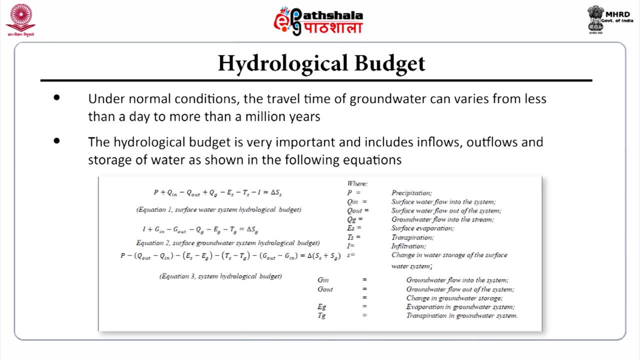 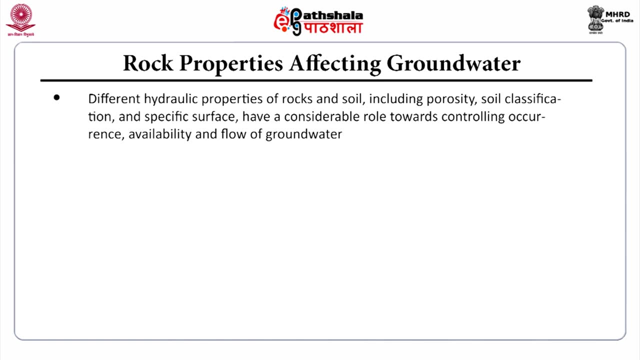 to more than a million years. The hydrological budget is very important and includes inflows, outflows and storage of water, as shown in the following equations: Rock properties: Different hydraulic properties of rock and soil, including porosity, soil classification and specific surface, have a considerable role towards controlling occurrence availability. 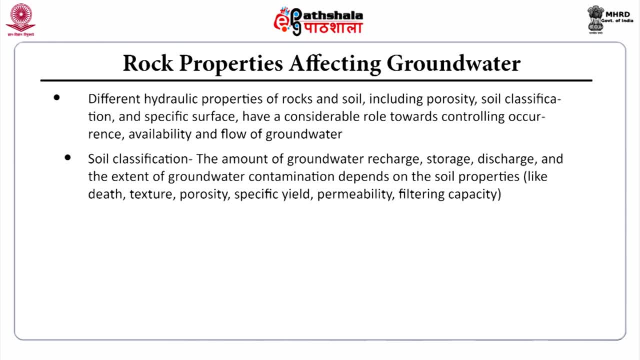 and flow of groundwater. Soil classification, The amount of groundwater recharge, storage, discharge and the extent of groundwater contamination depends on the soil properties like texture, porosity, specific yield, permeability, soil permeability and filtering capacity, Specific surface and specific yield. 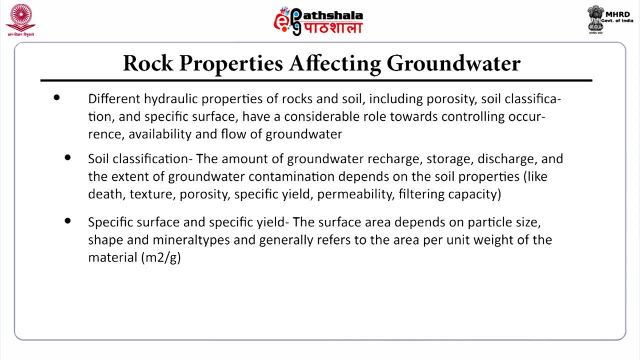 The surface area depends on particle size, shape and mineral types and generally refers to the area per unit weight of the material. Specific yield is the ratio of volume of water that could drain out from saturated rock to the total volume of rock, Now porosity. 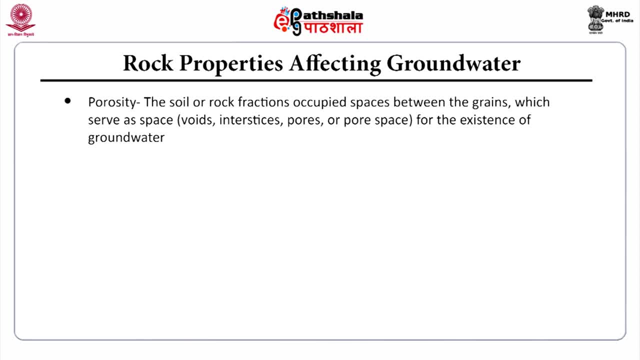 The soil or rock fractions. occupied Soil classification: Occupied spaces between the grains which serve as space for the existence of groundwater. These such openings are of great interest of hydrologists. The openings of rocks act as a reservoir of groundwater. Now permeability. 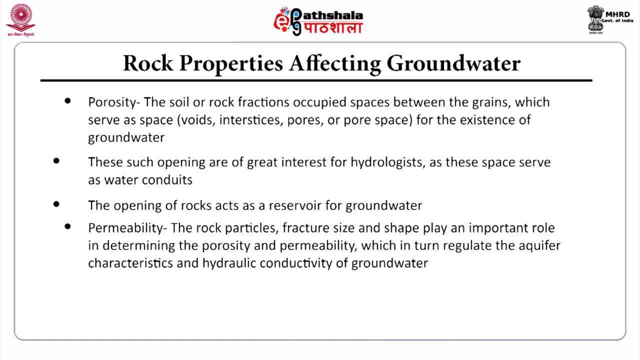 The rock particles, fracture, size and shape plays an important role in determining the porosity and permeability, Which, in turn regulate the aquifer Soil classification, Which in turn regulate the aquifer characteristics and hydraulic conductivity of groundwater. The permeability is the parameter which determines the ability of water transmission and movement. 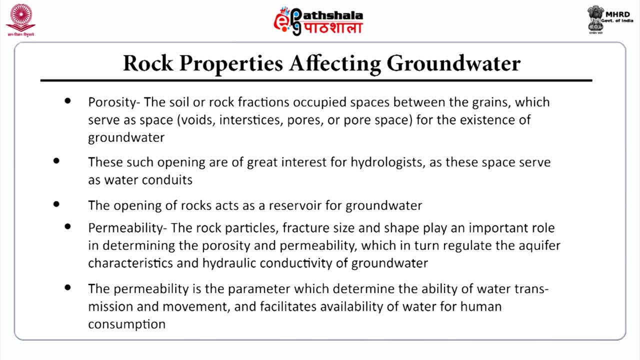 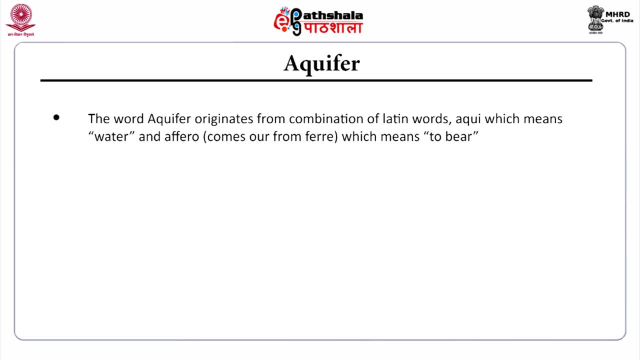 and facilitate availability of water for human consumption. Now we will discuss about aquifers. The word aquifer originates from a combination of two Latin words, equi, which means water, and ephro, Which means to bear. Lohmann in 1972 elaborates aquifers as geological formations which contains saturated permeable. 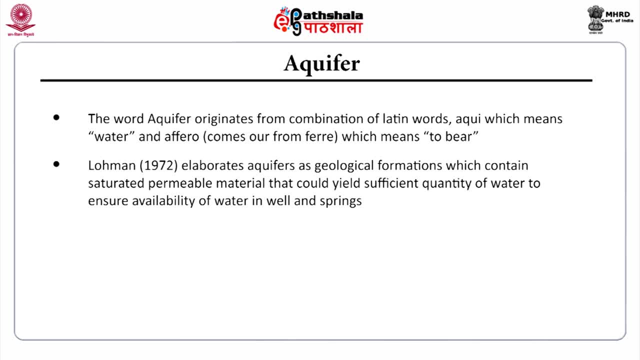 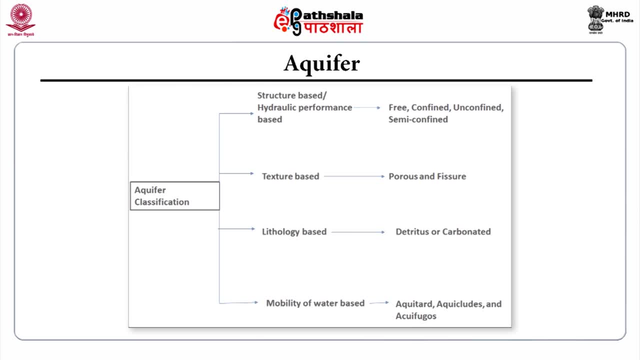 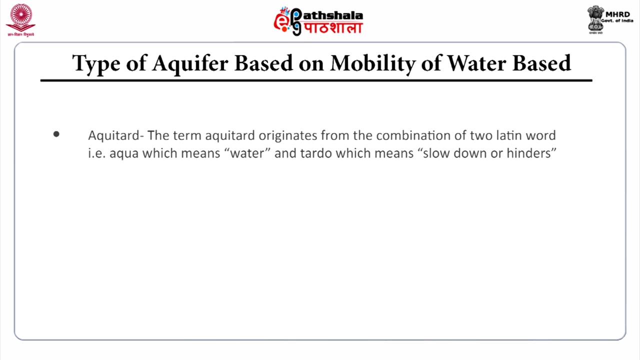 material that could yield sufficient quantity of water to ensure availability of water in well and springs. Aquifer classification: Aquifers can be classified depending upon the structure, texture, lithology and mobility of water based. Type of aquifer. based on mobility of water based. 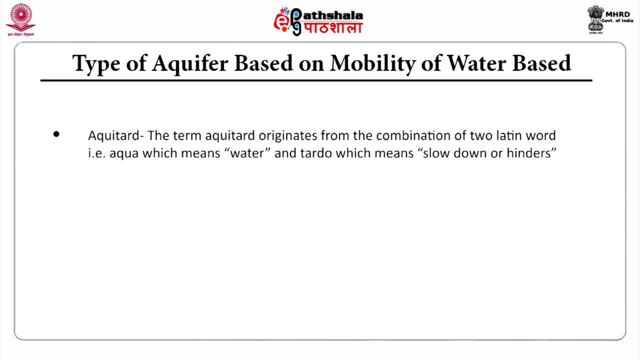 Equitard. The term equitard originates from the combination of two Latin words, equa, which means water, and tardo, which means slow down or hinders. Equitard represents the water saturated geological structures and confounding it to behave like resource for water supply. 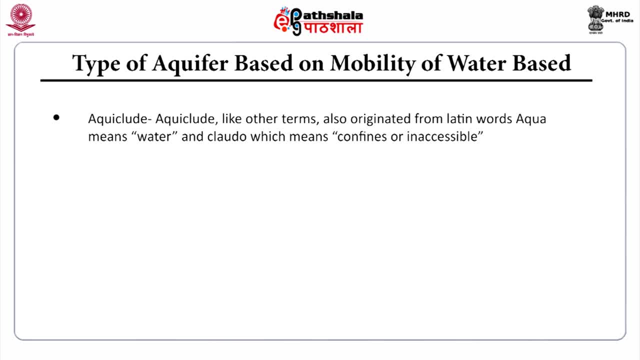 Equiclude, Equiclude. Equiclude, like other terms, also originated from Latin words equa means water and claudo means confines or inaccessible. An equiclude is solid, impermeable but porous structure underlying an aquifer. It defines as a water saturated geological unit that is incapable of transmitting significant. 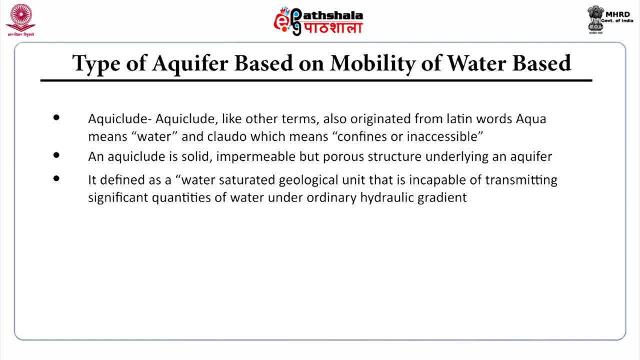 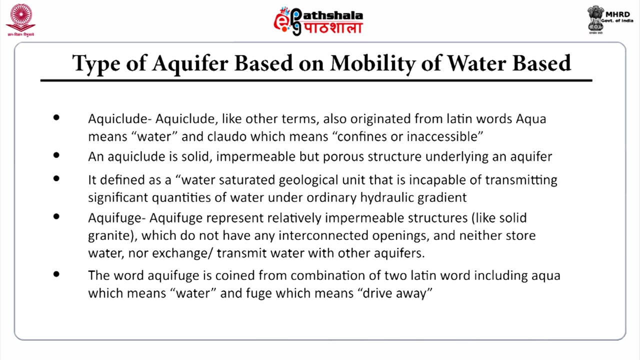 quantities of water under ordinary hydraulic gradient. Equiclude, Equiclude, Equifuse. Equifuse represents relatively impermeable structures which do not have any interconnected openings and neither store water nor exchange or transmit water with other aquifers. The word equifuse is coined from combination of two Latin word, including equa, which means 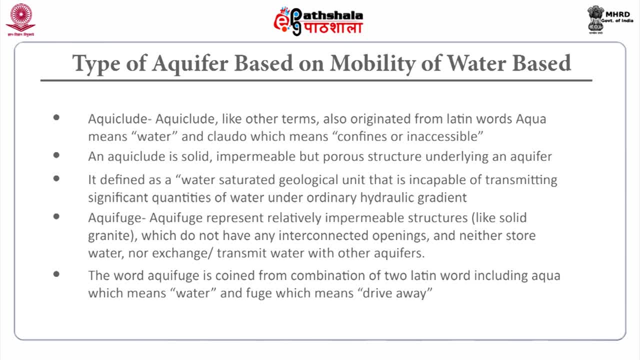 water and fuge, which means drive away. Types of aquifer based on structure. Okay, now we will discuss about various types of aquifer based on structure. Now we will discuss about three types of aquifers based on structure. 1. Defined Aquifer. 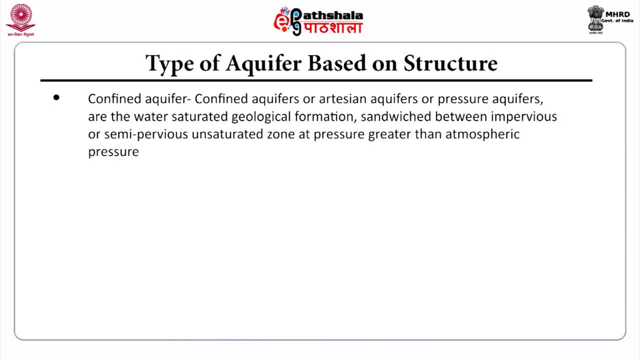 Defined aquifer or Artesian aquifer or pressure. aquifers are the water saturated geological formation sandwiched between imprevious or semi-previous unsaturated zone at pressure greater than atmospheric pressure. This pressure may sometimes results to rise in water level above earth's surface in wells. 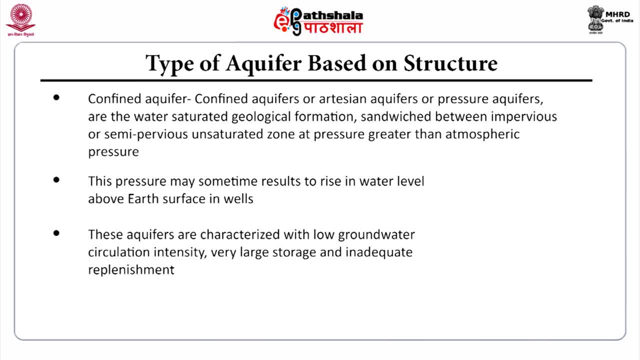 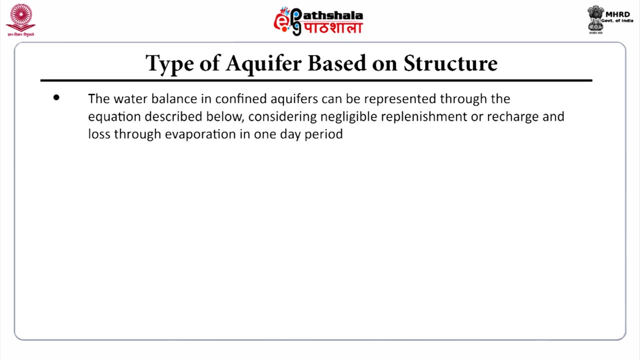 These aquifers are characterized with capillary growth or tear mass. 2. Atmospheric pressure: characterized with low groundwater circulation intensity, very large storage and inadequate replenishments. This figure shows about confined aquifers. The water balance in confined aquifers can be represented through the equation described. 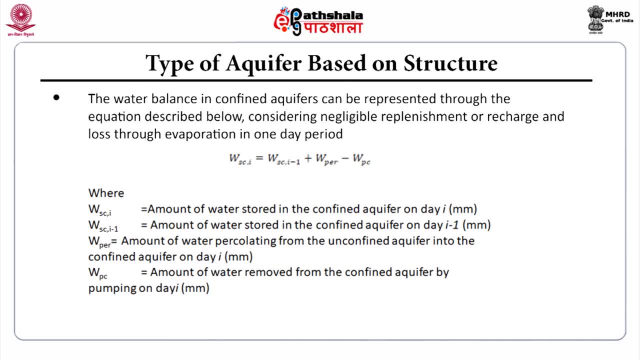 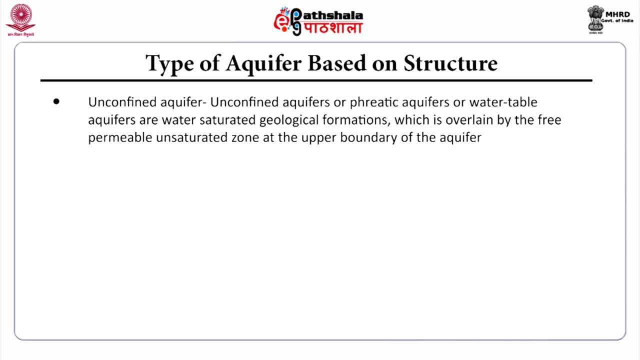 below, considering negligible replenishment or recharge or loss through evaporation in one day period. Unconfined aquifers are aquifers with water saturated geological formations which is overlaid by the free permeable unsaturated zone at the upper boundary of the aquifer. 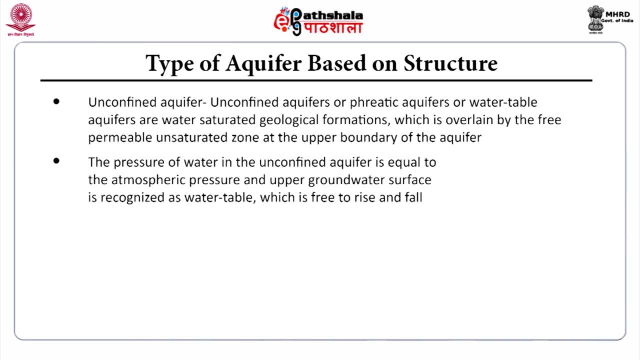 The pressure of water in the unconfined aquifer is equal to the atmospheric pressure, and upper groundwater surface is recognized as water table, which is free to rise and fall. Water does not rise above the water table in such aquifers. However, depth to the water table remain variable under various geological factors like topography. 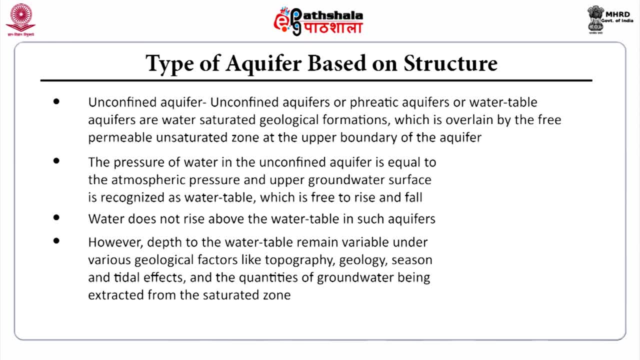 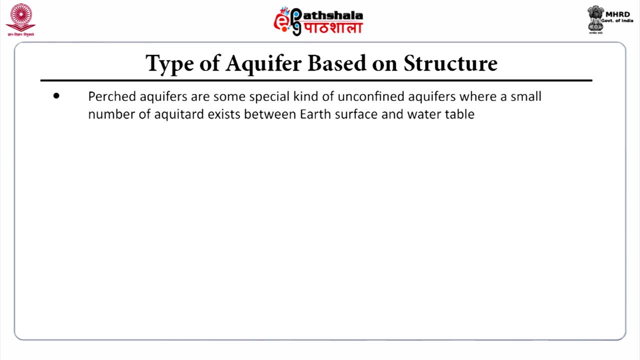 geology, season and tidal effects and the quantities of groundwater being extracted from the saturated zone. This figure shows about the unconfined aquifers. Perched aquifers are some special kind of unconfined aquifers where a small number of aquitards exist between our surface and water table. 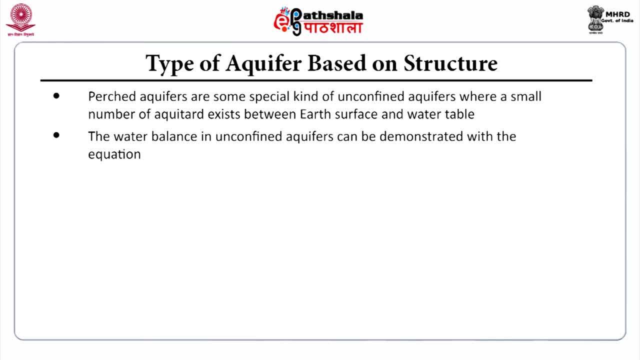 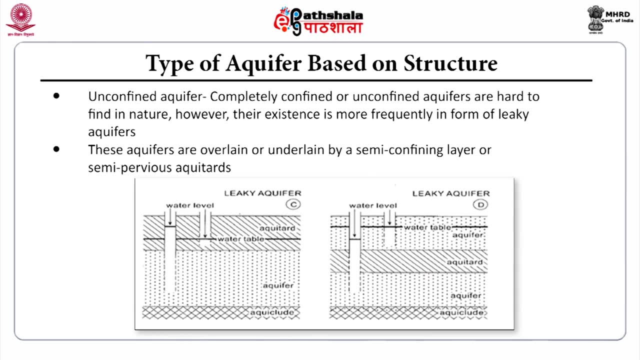 It is among the most common zombie health and fungal-containing grave sealant Deep. too many unsaturated source can be lead up to publiac–shell Emulsor have underline aquitard. then there is another aquifer and then there is aquiclude under that second aquifer. 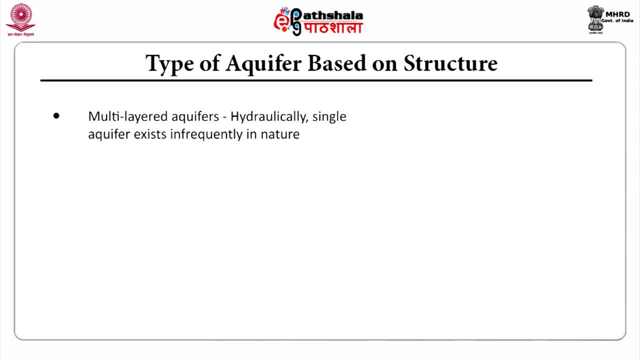 Multi-layered aquifers- Hydraulically single aquifer- exist infrequently in nature. Aquifer is a part of multiple aquifers which are arranged in a system. The movement of groundwater in such multi-layered aquifer system is much more complex than in the conventional way. 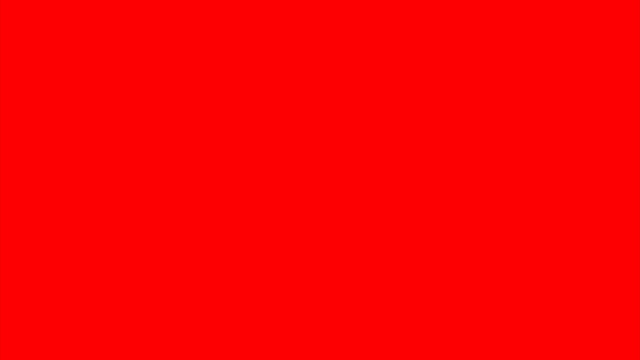 So the process of moving through a multi-layered aquifer system is as complex as a multi-layered aquifer system. Here's the flag. You can see the flag flying up and down the whole of the world. Can you see the flag?